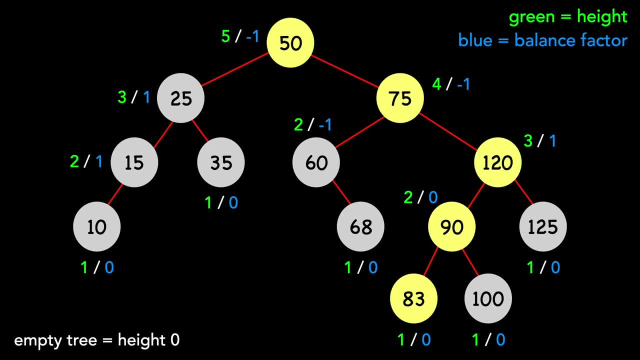 Its height is five, because there are five nodes on the path from 50 to 83.. To find its balance factor, we take the height of its left child minus the height of its right child. Three minus four is negative one. Please pause the video here if you need some time to review this. 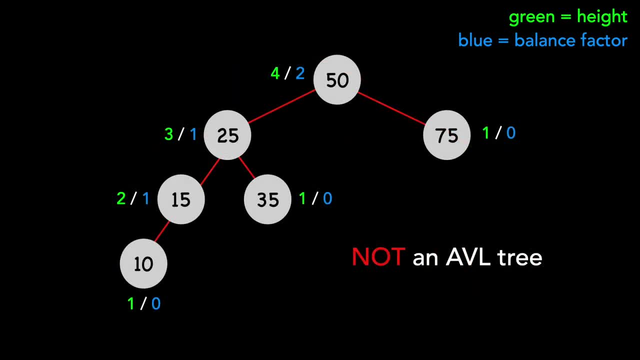 Here's an example of a tree that is not a green sub-tree, an AVL tree. As you can see, it has a node with a balance factor greater than one. Next, let's take a look at how AVL trees compare to red-black trees. 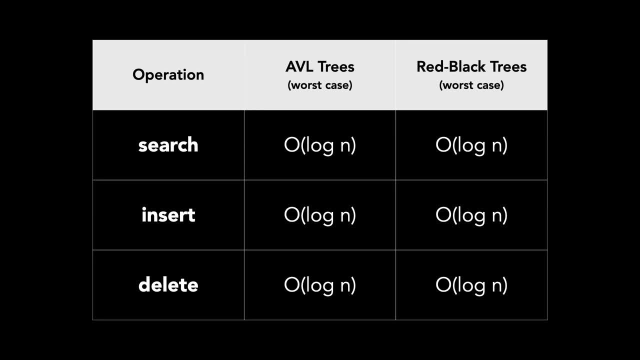 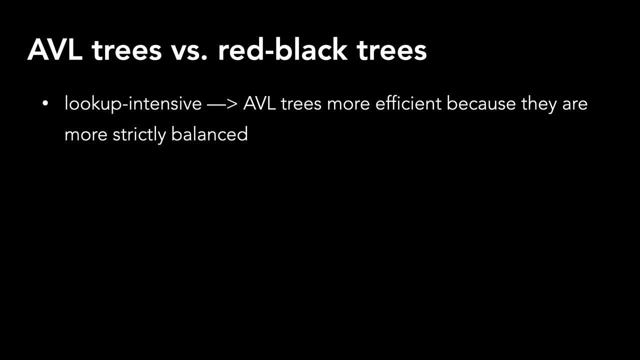 In the worst case, AVL trees and red-black trees have identical time complexities for search, insert and delete. However, for amortized time complexity, red-black trees have a time complexity of O for insert and delete. If your application is lookup intensive, AVL trees are more efficient because they 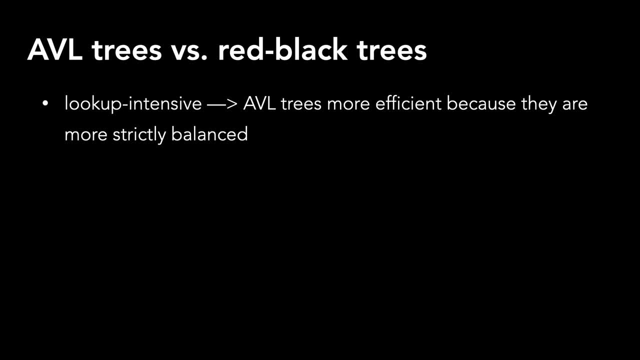 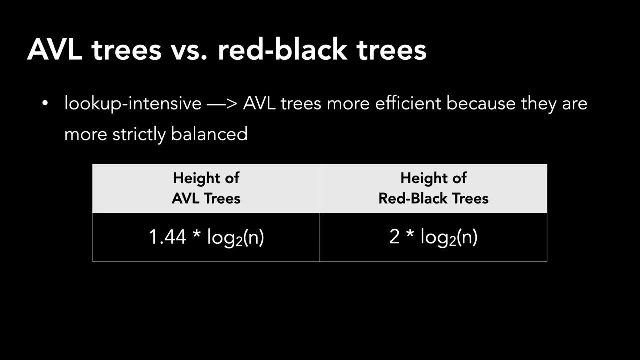 are more strictly balanced. That is, the height of an AVL tree is bounded by 1.44 times log base 2 of n, while red-black trees are bounded by 2 times log base 2 of n. Proving these values is outside the scope of this video. 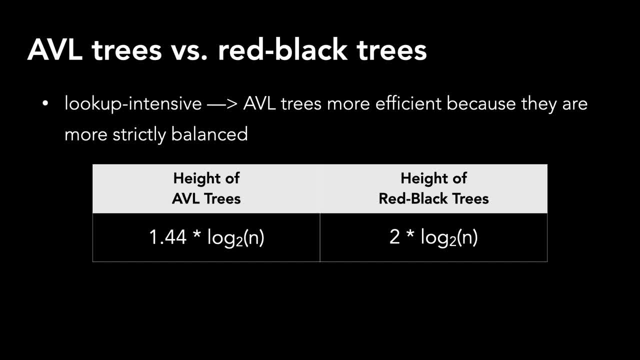 but I put links in the description. if you want to know more, I'll also link a paper from Ben Pfaff, who used to teach at the computer science department at Stanford, where he concluded that if insertions often occur in assorted order, AVL trees excel. 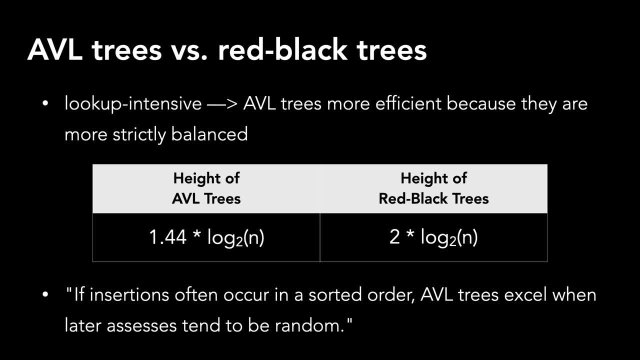 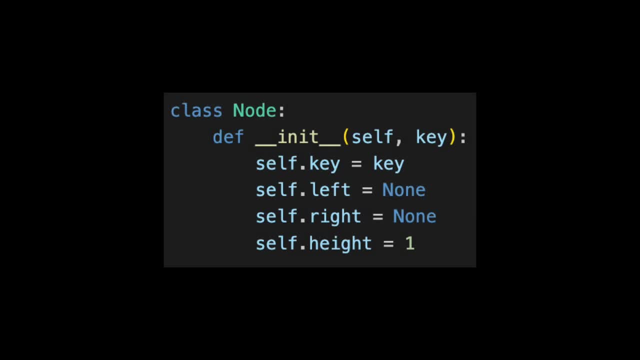 when later accesses tend to be random. Take a look at the paper if you're interested. He compares unbalanced binary search trees, AVL trees, red-black trees and splayed trees. Let's take a look at some code For our nodes. we'll hold the data in an attribute called key. 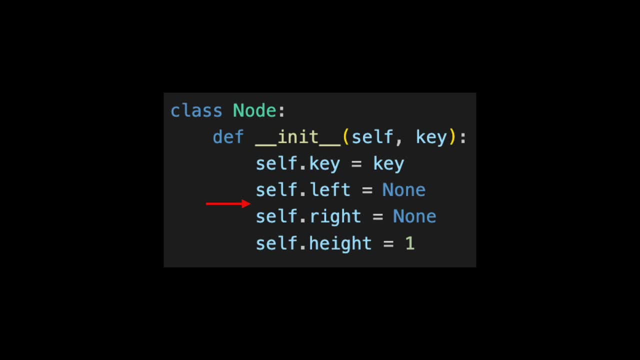 We maintain pointers to the left and right child and we also store the node's height, which is set to 1 upon creation. For the tree: we'll keep track of a pointer to the root node. For the tree: we'll keep track of a pointer to the root node.